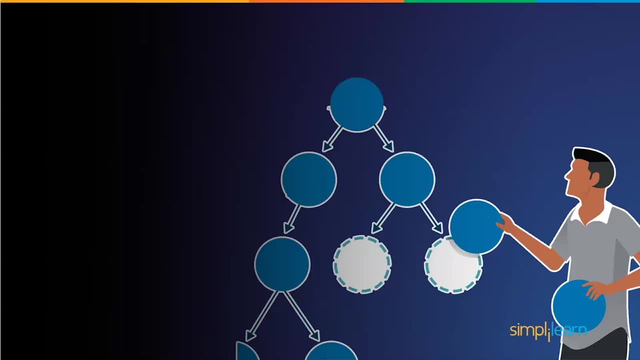 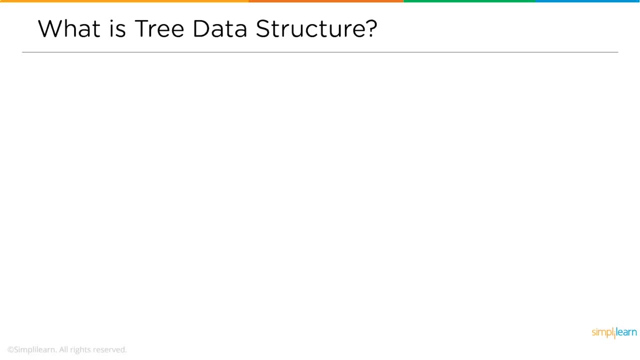 of trees in real time. I hope I made myself clear with the agenda. Now let's get started with the first topic, that is, what is a tree data structure? So what exactly is a tree data structure? The tree is a non-linear data structure. that. 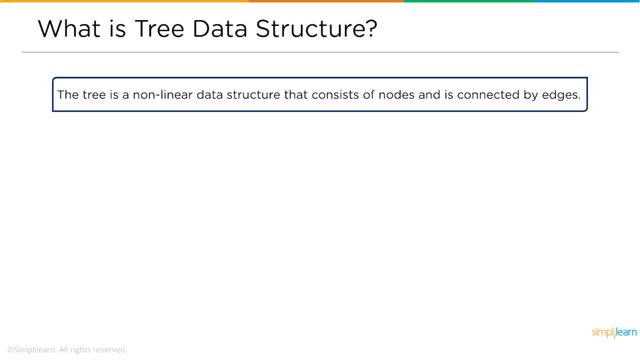 consists of nodes and is connected by edges. I know it's a little difficult to understand just by the definitions, So let me show you the pictorial chart and list of the non-linear data structures representation. As you can see, we have the elements, that is, 10, 20,, 30,, 40,, 50, 60 and 70. 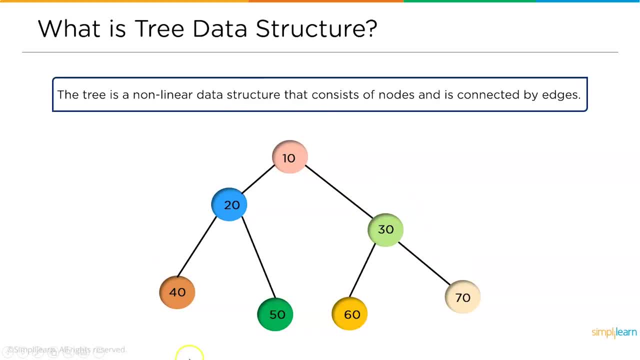 and all these are stored in the tree data structure. They are stored in a non-linear structure. If we had used arrays, it would have been in a linear, consecutive way where 10 starts first and 70 ends at the last position. Now, in the next section, we will discuss why we had made 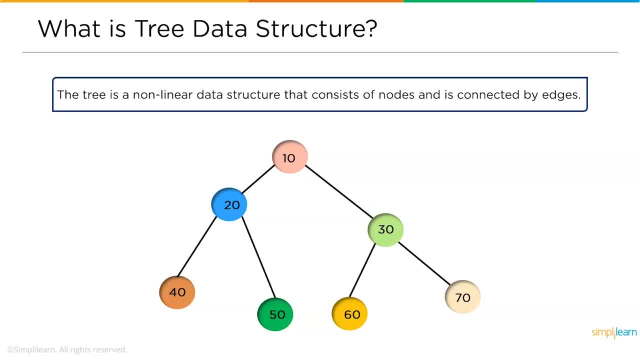 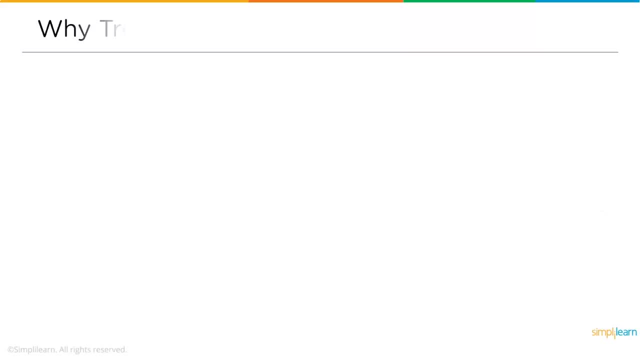 to a switch to the tree data structure when we already had a linear data structure, that is array, Now the next topic. that is why we need tree data structure. So there are many reasons why we had switched into tree data structure, and one of the reason is a. 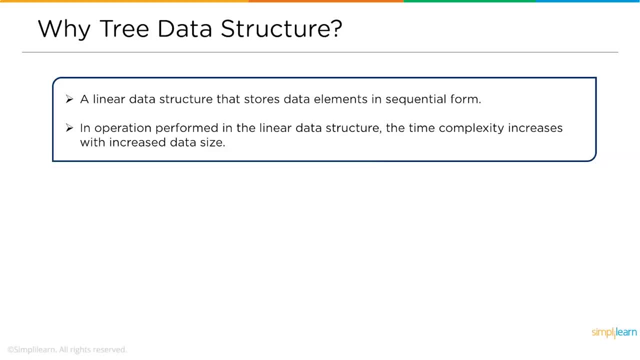 linear data structure always stores the elements in a sequential form, that is, one after the other, and in operations to be performed in linear data structure, the time complexity increases significantly. So in this case we have a tree data structure that is a linear data structure. as the data size increases, You can see here that, as discussed before, the elements are stored in a. 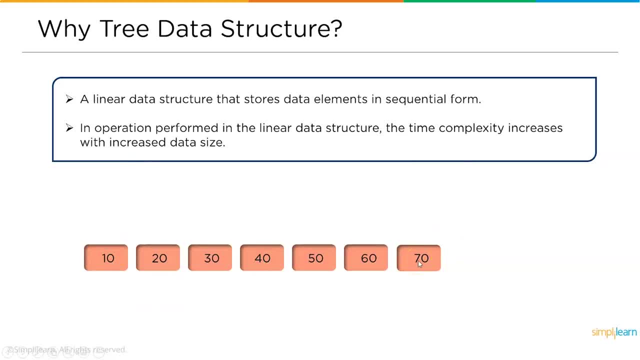 linear form that is 10 at the first place and 70 at the last place. Imagine you wanted to access the element 70. then, using the traversal, you had to start from the first position. that is, 10,, 20,, 30,, 40 and slowly at the end is 70. So accessing that particular element is really time consuming. 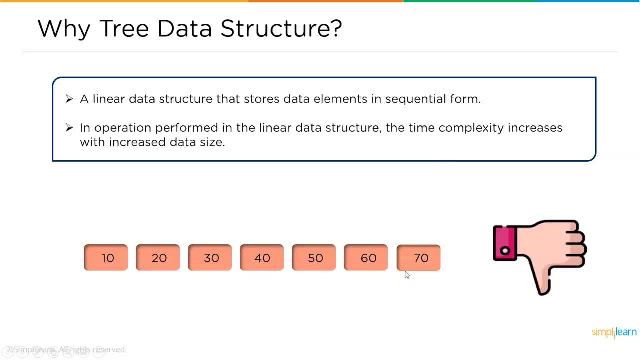 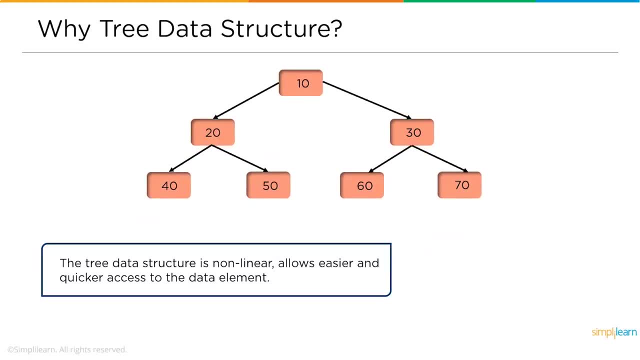 We are facing this just for 70 elements. Imagine if we had 700 elements, Right? So that is exactly why we had made a switch to tree data structure and using tree data structure. we have many advantages, as the tree data structure is completely non-linear and it allows easier 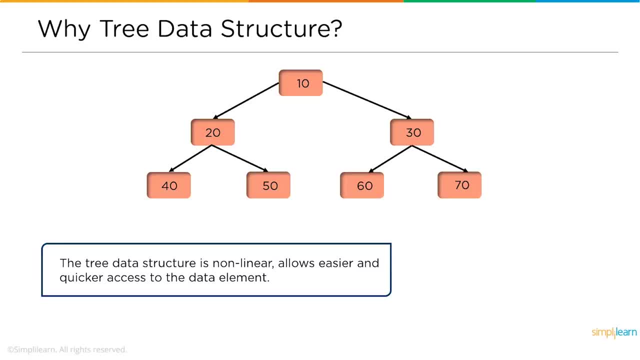 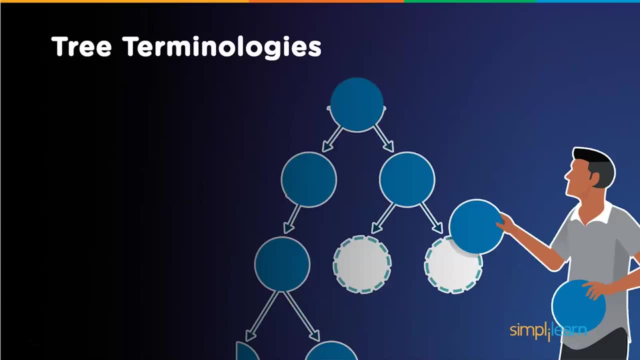 access and quicker access of the data elements. How is that possible? We will look into it into the next segment where we will discuss about the traversal of trees. Now, before we understand the traversal of trees, we should understand another important topic, that is, the terminologies of tree. 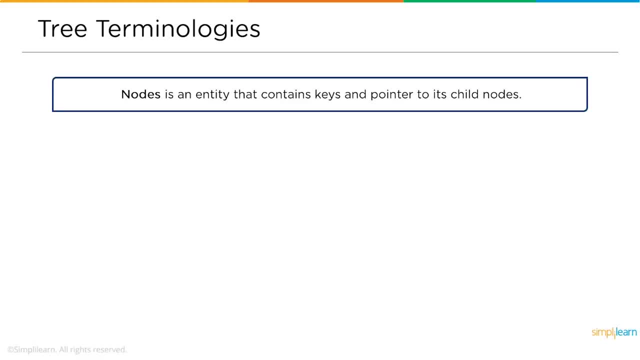 So the first one is the node. Node is the entity that contains the keys and pointer to its child nodes. So here you can see that the elements a, b, c, d, e, f and g are the elements. So each and 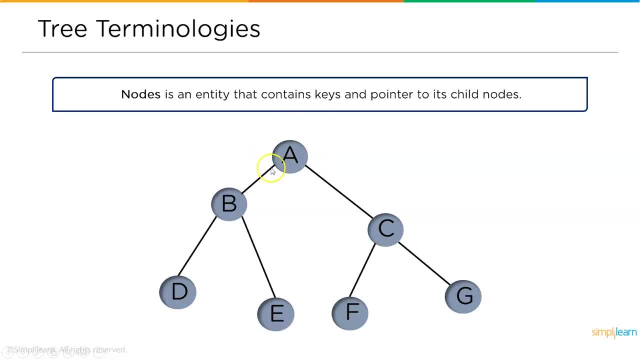 every element or the blue dot is called as a node, and the blue dots here are 1,, 2,, 3,, 4,, 5,, 6 and 7.. So we have seven blue dots. So we have seven blue dots, and we have seven blue dots, and we have seven. 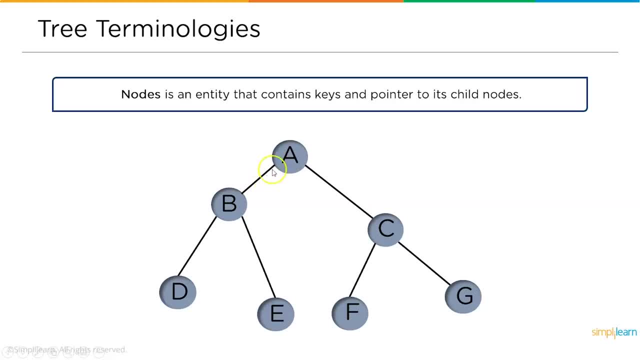 elements here. So you can see the line between each elements right. So this particular line is called edge. Now we will discuss about the edge in the next part. So the connecting links between any two nodes are called as edges. So we discussed about the nodes right where the element is stored. 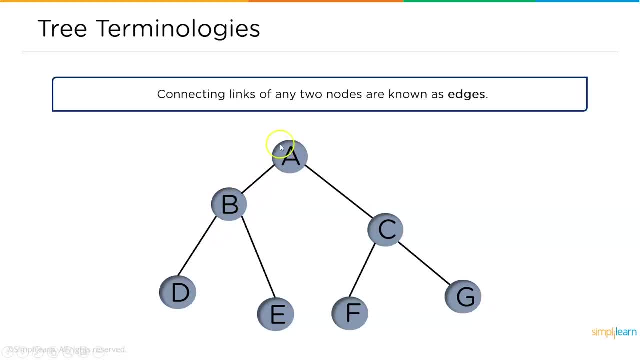 the blue dots are the nodes and the lines connecting between the elements or nodes is called as the edge. So out of all the nodes, this first node, that is, the element a, is called as the root node in a tree data structure. So indirectly root node. 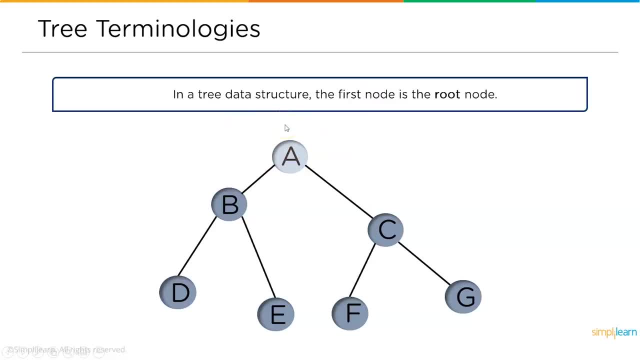 is also called as the parent node of all the nodes. Now we will understand what are parent nodes and children nodes. So in a tree data structure, the node that is the nodes predecessor is called as parent node. So here we have discussed that a or the root node is the 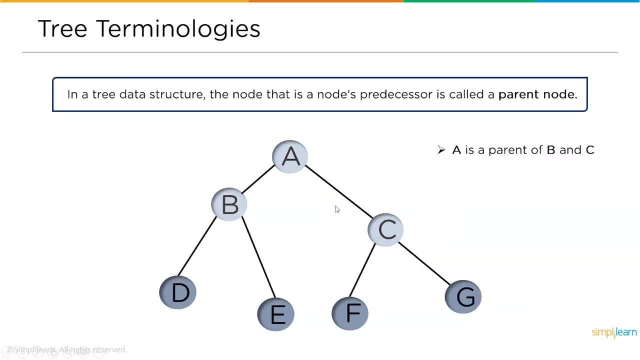 parent of all nodes. So for a, b and c nodes are children nodes and for B and C nodes A happens to be the parent node. Similarly, D and E are the children nodes of B, and F and G are children nodes of C and the nodes D and E have B as a parent node and the 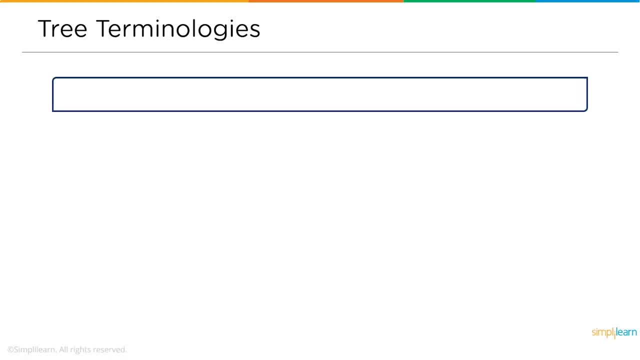 nodes F and G have C as the parent node. Now, followed by that, we will understand the descendant node. So, as discussed before, the descendant node is the node that comes after the parent node. Here the B and C are the descendants of A and D and E are descendants of B and similarly. 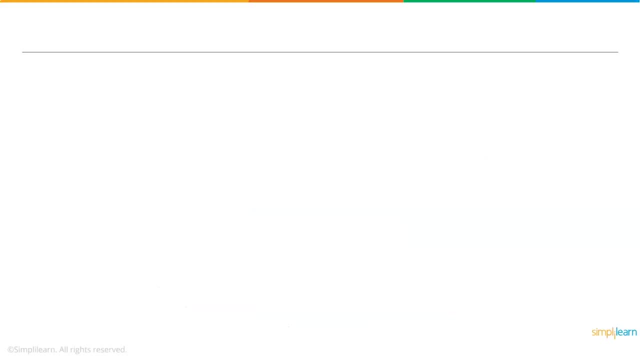 F and G are the descendants or children of the node C. So in a tree data structure the node which does not have any child is called as the leaf node. Now at the end we have D, E, F and G. So these particular nodes do not have any children, nodes like B and C. So 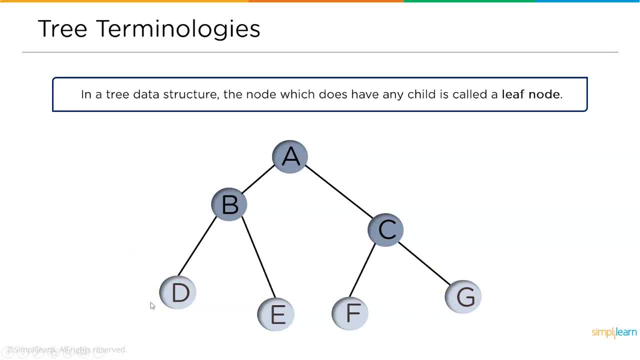 these particular four nodes which do not have any children are called the children nodes here. the internal nodes are B and C, which have at least one child In a tree the total number of children of a node are called as the degree of that node. So in this particular diagram 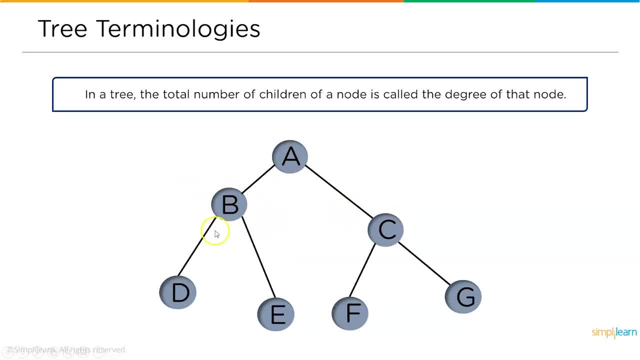 the degree of a root node is 2 because it has two child nodes and the degree of B is 2 as it has two child nodes. So in this particular diagram, the degree of a root node is 2 because it has. Similarly, the degree of C is 2 because it has 2 child nodes. 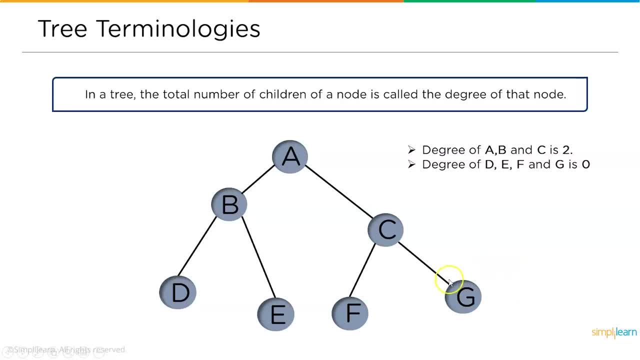 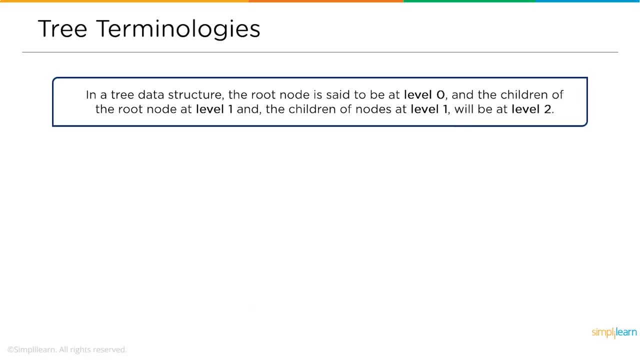 But when it comes to D, E, F and G, the degree is 0 because they do not have any child nodes In a tree data structure. the root node is said to be at level 0 and the children of the root node are said to be at level 1, and the children nodes of the level 1 are at level 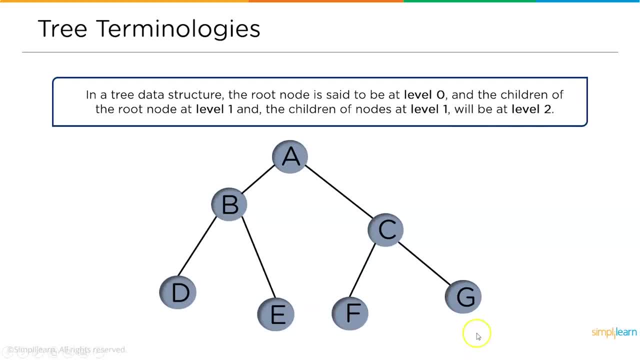 2.. So to understand this, let us go through the diagram. As you can see, this particular root node is called as level 0, and followed by that we have the children nodes of A, that is, B and C, and that level is called as level 1. 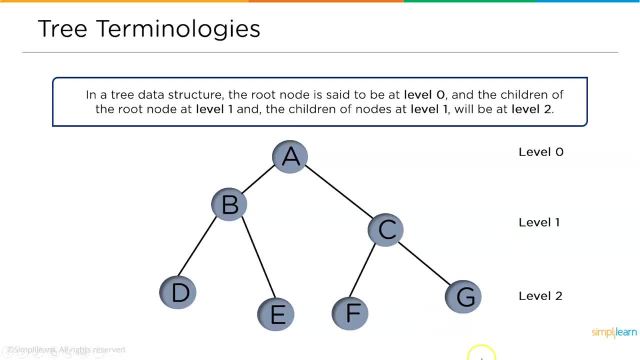 and followed by that we have level 2, and if this tree goes forward, the levels also increase accordingly. Now in a tree data structure, the total number of edges from a leaf node to the particular node is the longest path, and this particular path is called as the highest path. 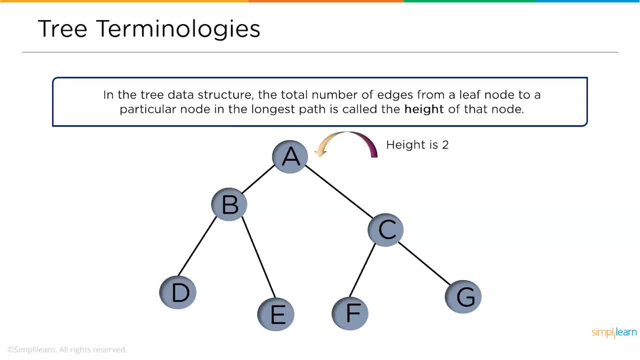 The height of that node. Now here we have our general tree data structure and here you can see: the height of node A is 2 and the height of node B and C together is at 1, and the height of the last leaf nodes happens to be 0.. 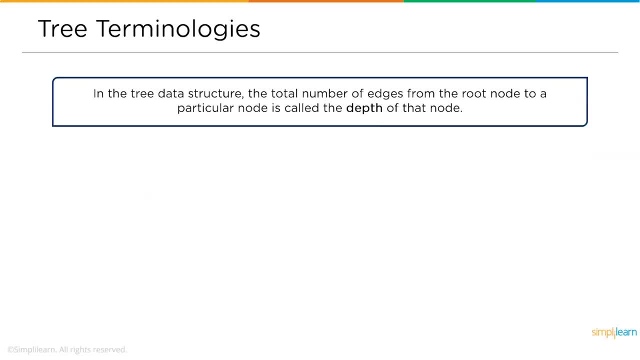 Next, in the tree data structure, the total number of edges from the root node to a particular node is called as the depth of that node. Now, in this particular tree data structure, The depth of the root node is 0 and the depth of B and C together is 1, because the number 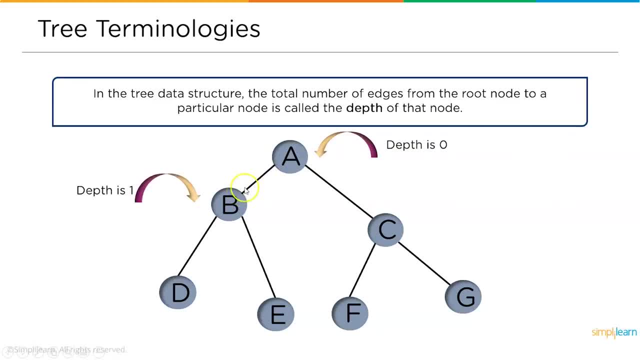 of edges connecting to the node A from B is just 1 and similarly the number of edges connecting the node C from A is just 1.. So the depth of both B and C is 1.. Now if we consider the last leaf nodes, then the depth is 2 because, if you see, G is connected. 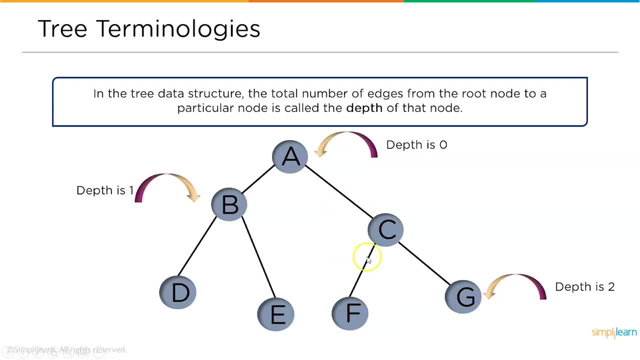 to A using two different edges. Similarly, F is connected to A using two different edges and E and D also have two nodes to connect to A. So the depth is 2.. Now in the next segment we will understand the tree node. 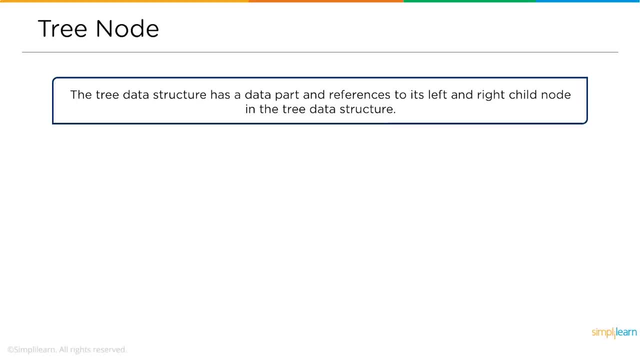 So the tree data structure has data part and references towards left and right child node in the tree data structure. So here you can see this is the node and the node has three segments, That is, data element and the references towards left, the child and the references towards 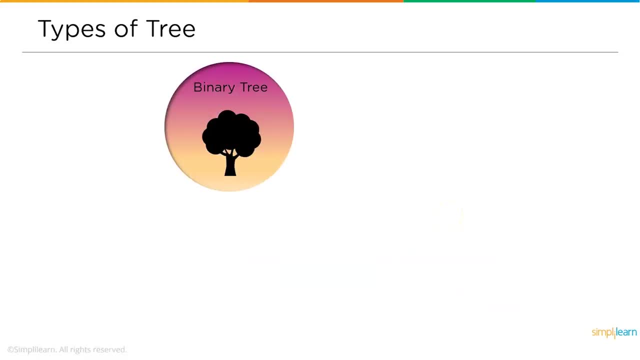 right child. Now there are four different types of trees. The first one is the binary tree, followed by that we have the binary search tree, Then we have AVL tree and finally we have the B tree. Let us discuss each one of them. 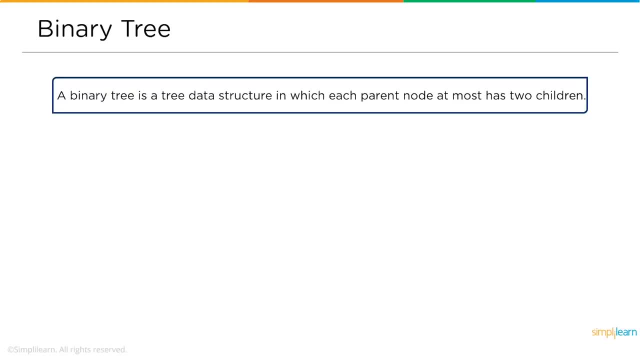 The first one is the binary tree. A binary tree is a tree data structure in which each parent node at most has two children. So in this particular tree will have at most two children. That means it might have one or more than one, but not more than two children per node. 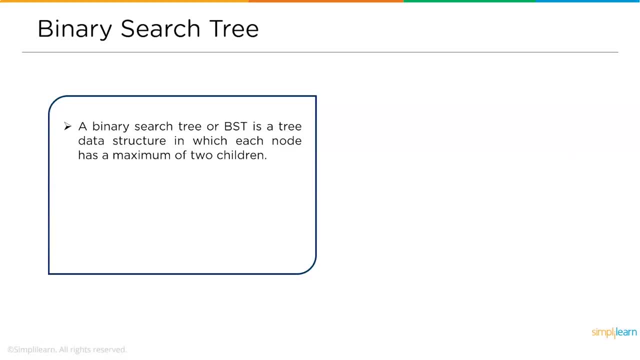 Moving ahead. we have the binary search tree. So a binary search tree, or a BST, is a tree data structure in which each node has a maximum of two children. All nodes of the left sub-tree are less than the right node. All nodes on the right sub-tree are more than the root node. 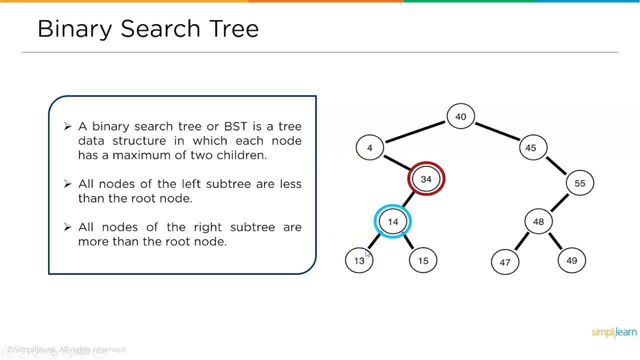 So here you can see the image, or the GIF, which represents the image of a binary search tree. So here all the nodes of the left sub-tree are less than the root node and all the nodes of the right sub-tree are more than the root node. 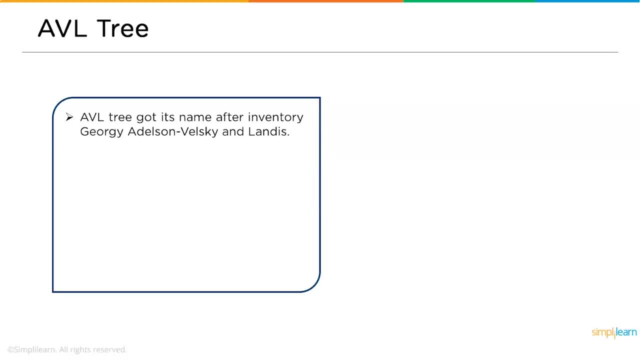 The next type of the tree is the AVL tree. The AVL tree got its name after Inventory Georgie, Adelson, Welsky and Landis. AVL tree is the self-balancing tree in which each node maintains a balanced factor whose value is either 1,, 0 or minus 1.. 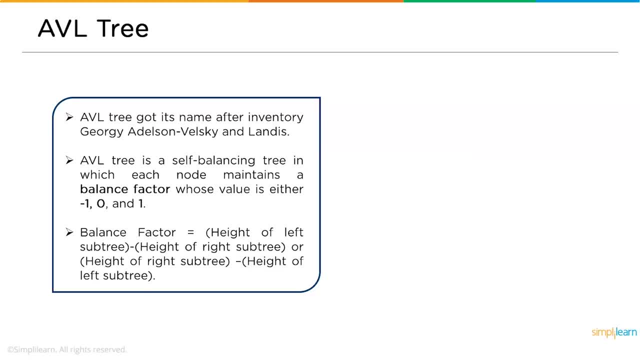 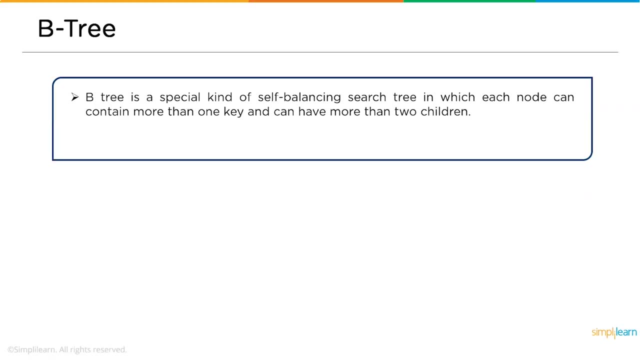 Balanced factor is equals to height of the left sub-tree minus height of the right sub-tree, or height of the right sub-tree minus height of the left sub-tree. So in this particular image you can identify it as an AVL tree. And now the last type of tree, that is, the B tree. 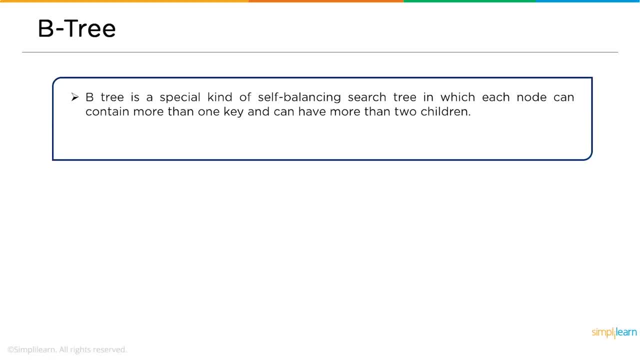 B tree is a special kind of self-balancing search tree in which each node can contain more than one key and can have more than two children. B tree is also known as the height-balanced M-way tree. Now, in this particular GIF, we can see how a B tree looks like. 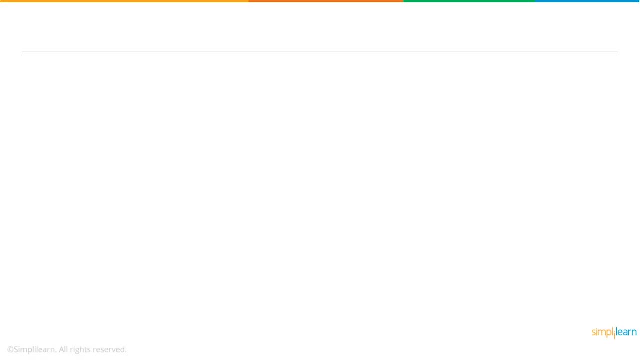 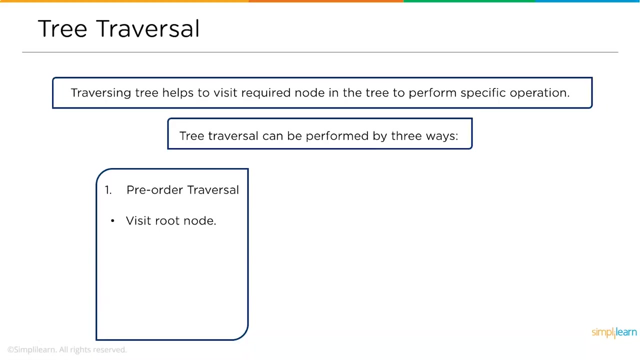 Now, followed by this, we will discuss the tree traversal. So traversing a tree helps to visit required node in the tree to perform specific operations. Tree traversal can be performed in three different ways. The first one is the pre-order traversal, Where we visit the node and visit all the node from the left side, then visit all the. 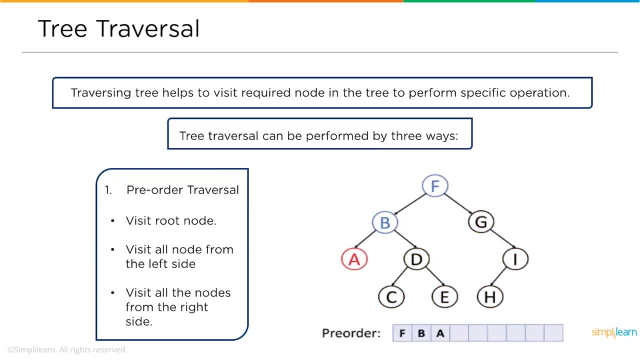 nodes from the right side. So this particular GIF is an example for pre-order traversal, where we visit all the left side nodes first, then we visit the right side nodes. Now we will move ahead into the next type of traversal, that is, the in-order traversal. 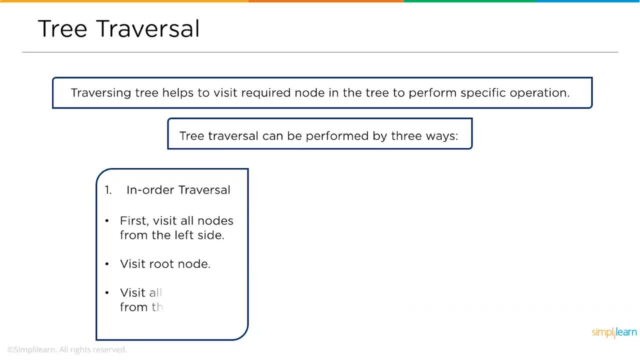 First we visit all the nodes from the left side, then we visit the root node and then we visit all the nodes from the right side. So this particular GIF will be an example for the in-order traversal, where we visit all the left side nodes, then we visit the root node and followed by that we will visit 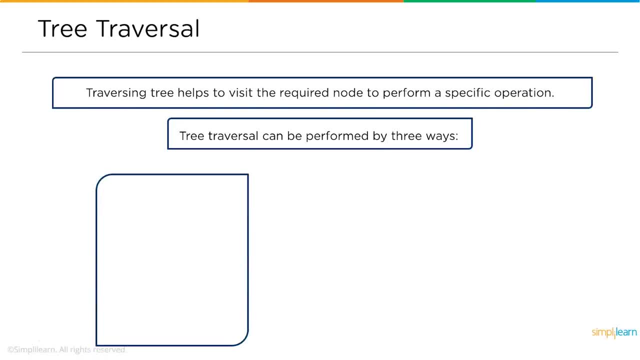 the right side nodes. And the last type of traversal is the post-order traversal, where we visit all the nodes from the left side first, then we visit all the nodes from the right side and finally visit the root node. So this particular image on the right side is an example for post-order traversal.